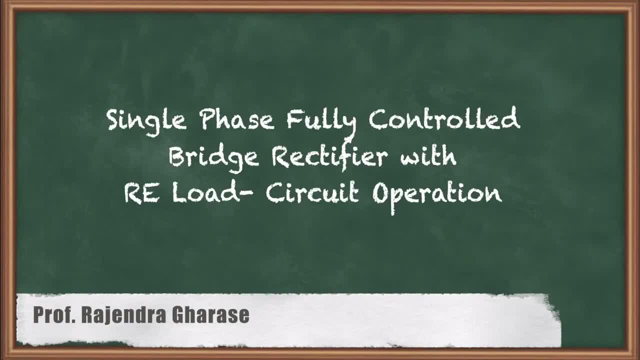 Hello friends, in this video we are going to discuss the circuit operation of single phase full wave controlled rectifier, fully controlled bridge configuration and the load is RE load. RE load is nothing but the battery charging circuit. We have already discussed this type of load in the center tapped transformer configuration, So let us discuss what is the change. 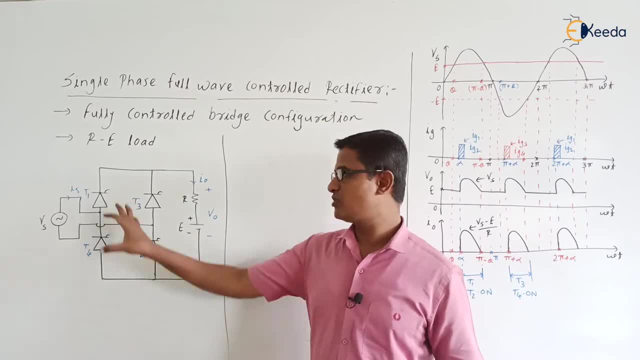 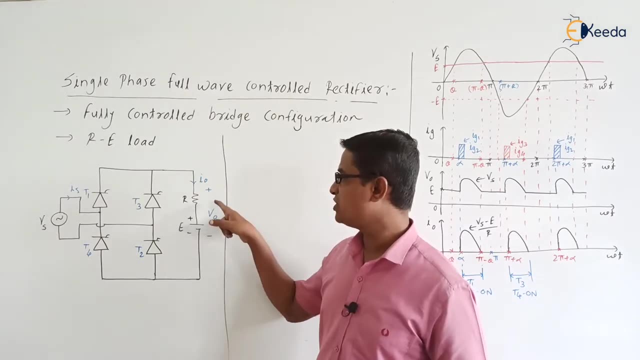 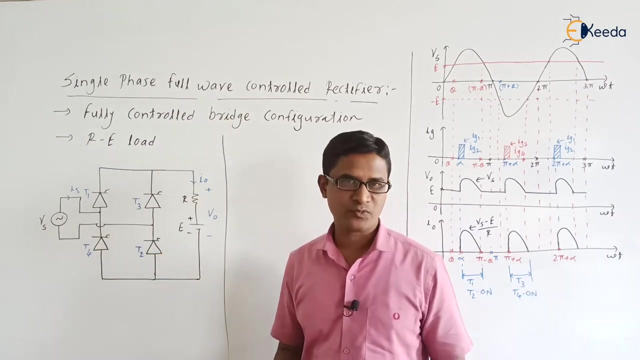 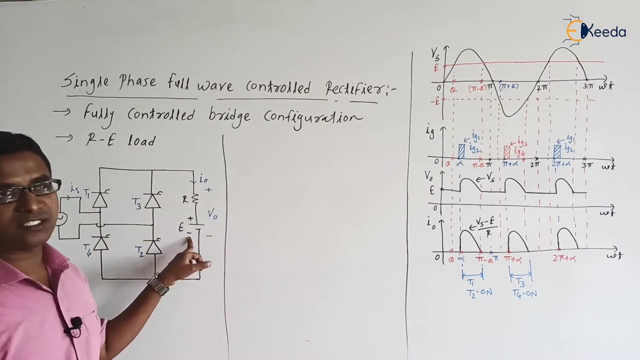 So here it is the circuit diagram. We are using the four switches. VS is the supply voltage and the load is RE. So voltage across load is V0, current flowing through the load is I0.. So next, supply voltage VS is having a positive value as well as negative value. 0 to pi VS is positive, pi to 2 pi VS is negative And in the load we are having the emf, that is the battery magnitude, emf of the battery. 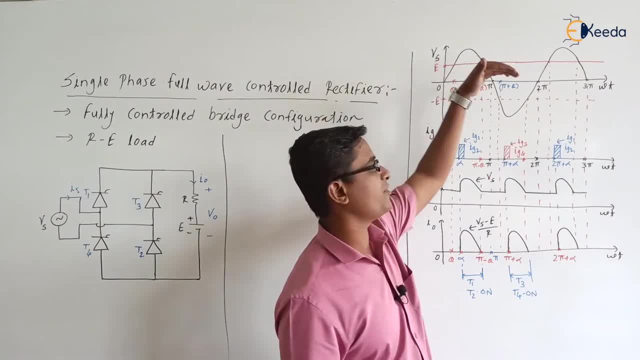 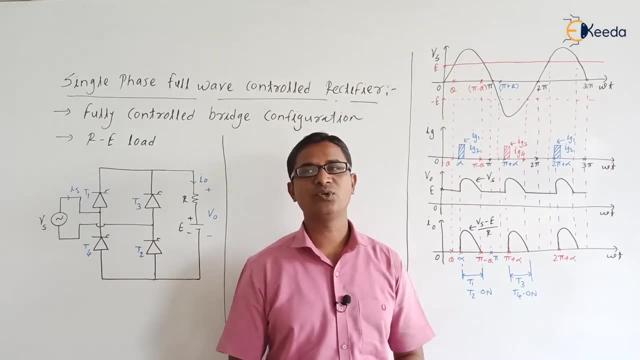 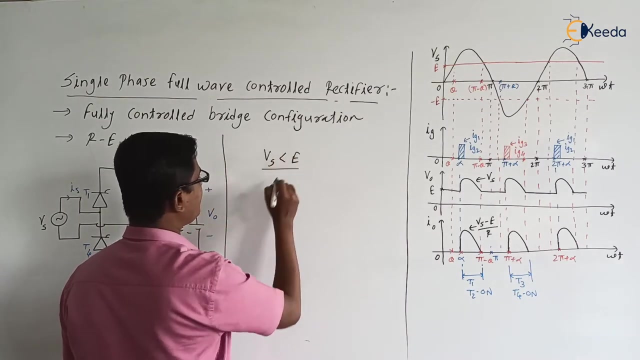 So here it is a VS we are having And here it is the emf. okay, so during omega t is equal to 0 to theta, right. during omega t is equal to 0 to theta. okay. vs is less than e right for the interval. vs less than e right vs less than e. okay, our. 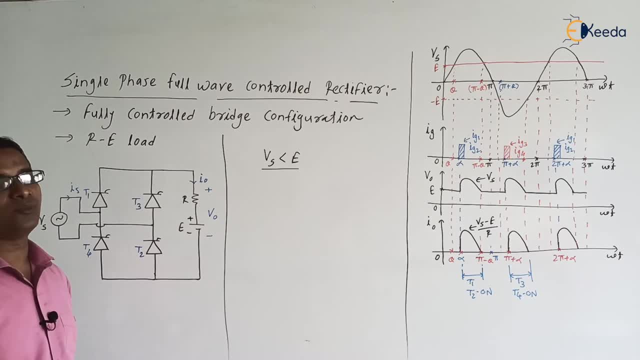 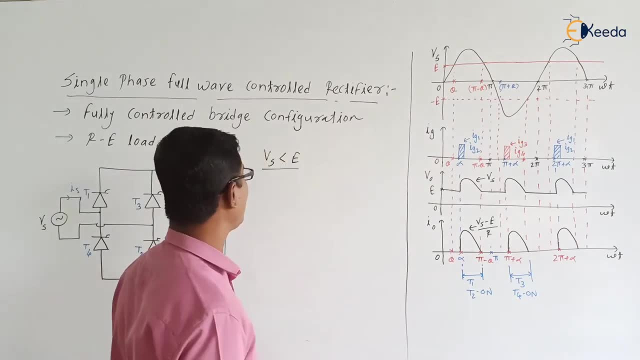 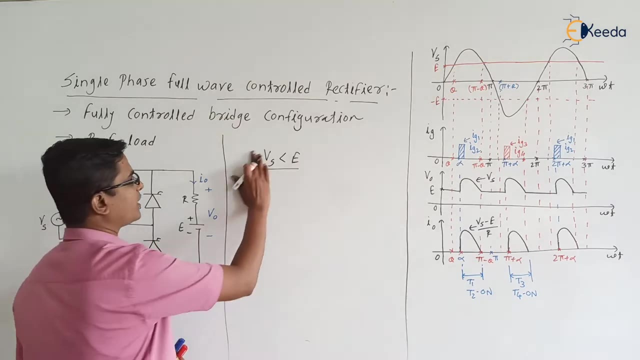 thyristors. respective thyristors will be in the reverse blocking mode. right, those will be in the reverse bias mode. okay, so that is for omega. t is equal to 0 to theta. right for 0 to theta. yes, vs is less than e. if supply voltage is less than e, okay, from 0 to theta. right, so we can write it as: 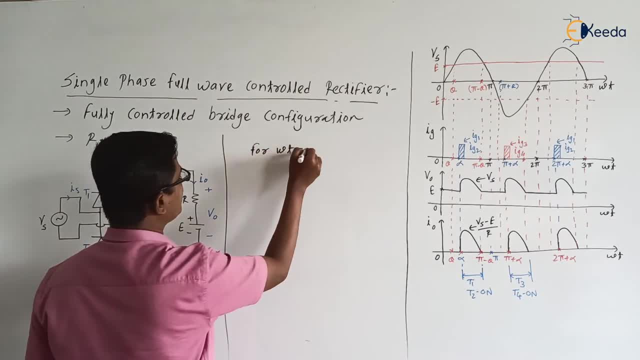 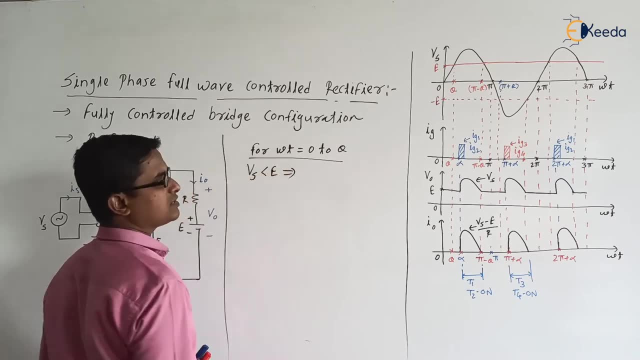 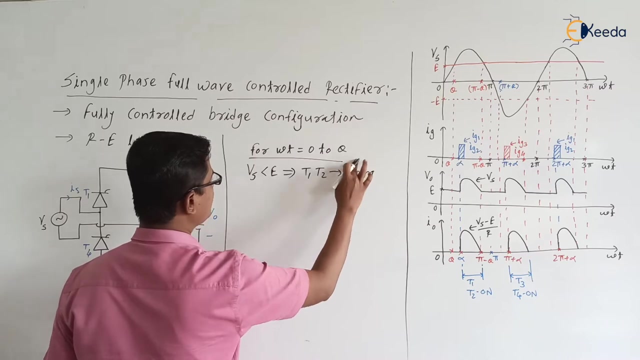 a for omega t is equal to 0 to theta. 0 to theta. yes, vs is less than e. right, vs is less than e. so thyristor t1, t2: yes, these two thyristors will be in the forward blocking mode, right, sorry, reverse. 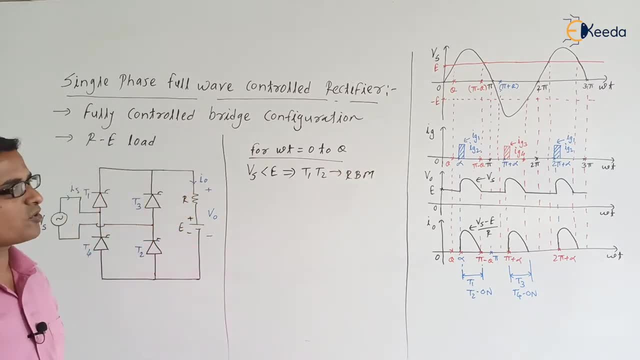 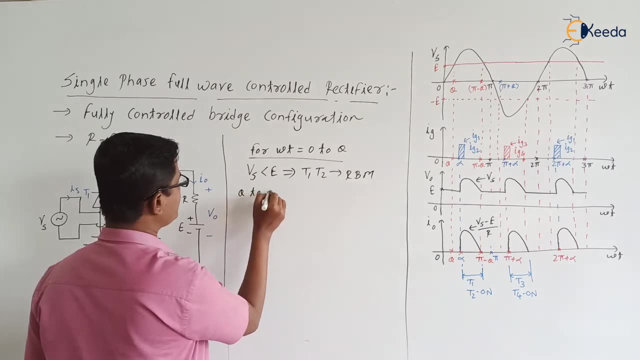 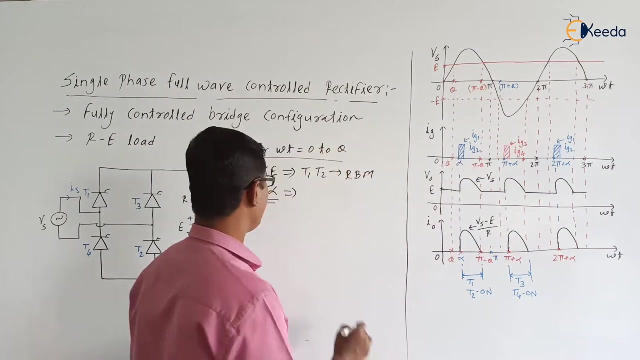 blocking mode. those two will be in the reverse blocking mode, right, because vs is less than e. okay, next, from theta to pi plus alpha. sorry, theta to alpha. from omega t is equal to theta to alpha. during theta to alpha. yes, what will happen? from theta to alpha? yes, vs is greater than e. yes, we. 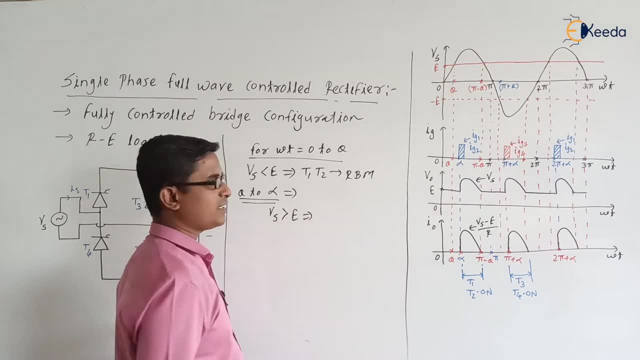 can write it as a vs greater than e. if vs is greater than e, our thyristors t1- t2 will be in the forward blocking mode right. vs greater than e means what thyristor anode voltage will be greater than the cathode voltage. right, because when circuit is at the raised position then the 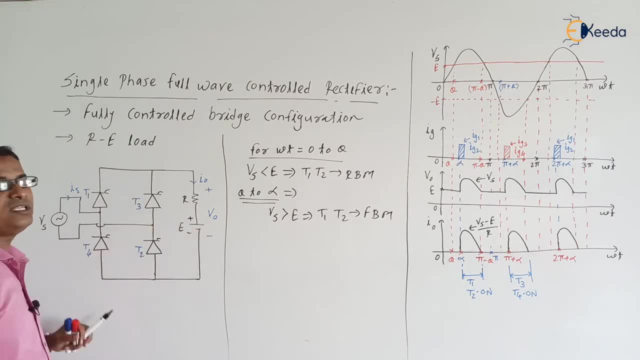 voltage that will be appearing at v0 is nothing but the e. okay, so therefore, t1, t2 will be in the forward blocking mode. okay. and after pi, after alpha, what will happen? yes, thyristor, t1, t2 will be in the conduction mode. so here, t1, t2 will be in the conduction mode. the conduction will be yes. 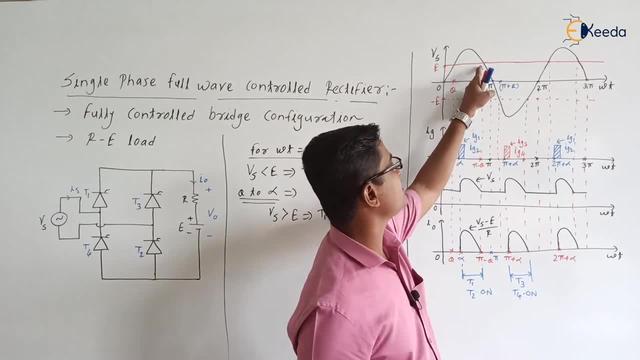 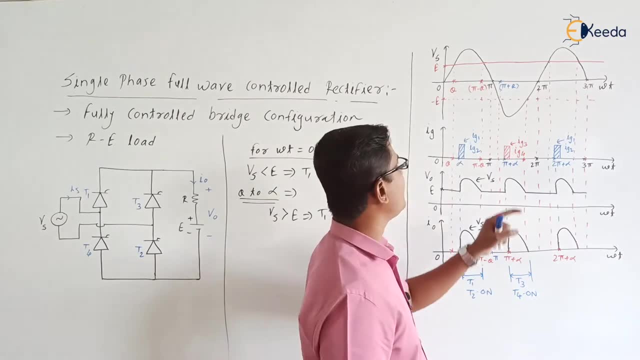 from alpha to till the instant at which vs is greater than e. right, if you check, after pi minus theta, vs is less than e. okay, so if vs is less than e, then what will happen? yes, thyristor t1, t2 will be in the again. 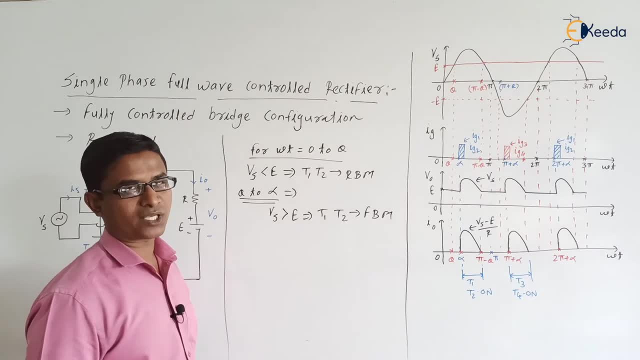 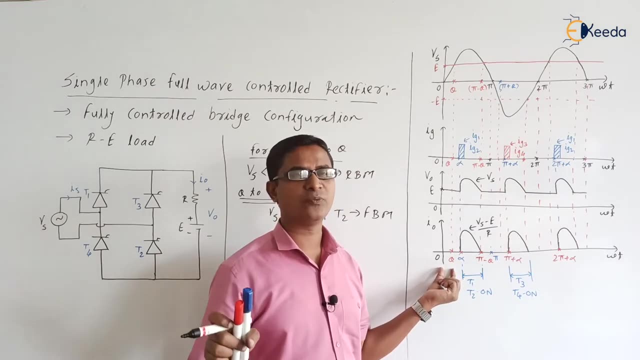 switches from forward conduction to the reverse blocking, forward conduction to the reverse blocking. are you getting the point? okay? so from 0 to theta, the mode of operation of thyristor t1, t2- it is in the reverse blocking mode, 0 to theta. theta to alpha. forward blocking mode, alpha to. 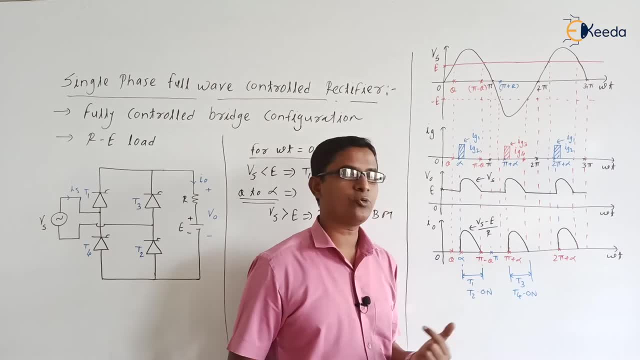 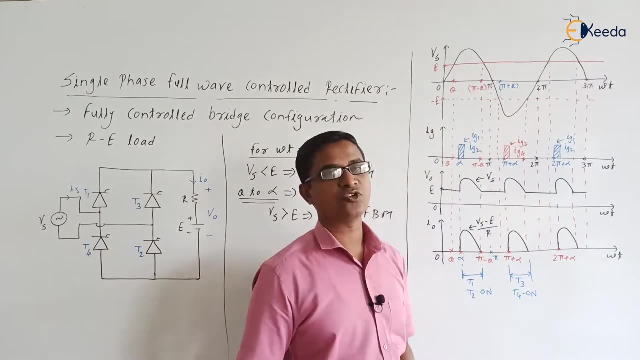 pi minus theta, forward conduction mode: pi minus theta to pi. yes, it is the reverse blocking mode. are you getting the point? okay, and similarly for the second negative half cycle: okay, so when supply is negative, yes, we are having the thyristor t3, t4. 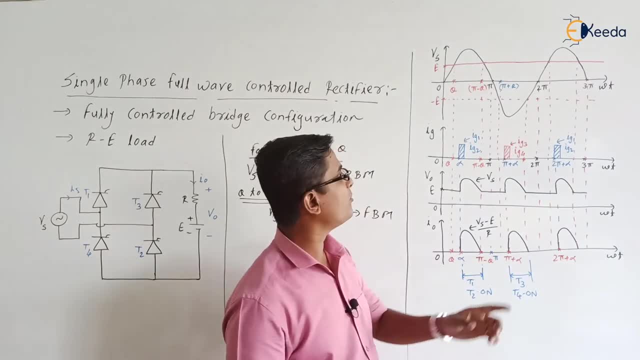 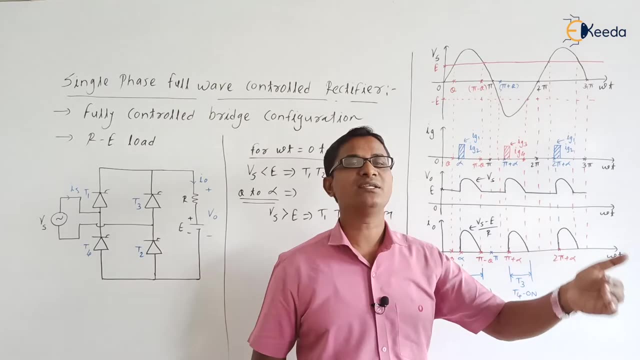 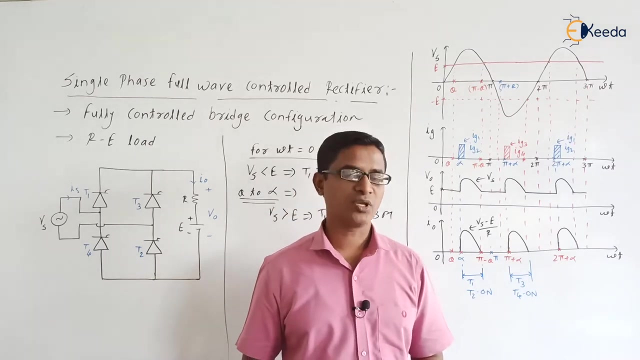 okay, will be in the forward bias mode. but yes, from pi to pi plus theta means during this interval: okay, vs is less than e, right, vs is less than minus e okay. so due to that, from pi to pi plus theta, our thyristors t3, t4 will be in the reverse blocking mode. okay, next, pi plus theta to 2 pi. 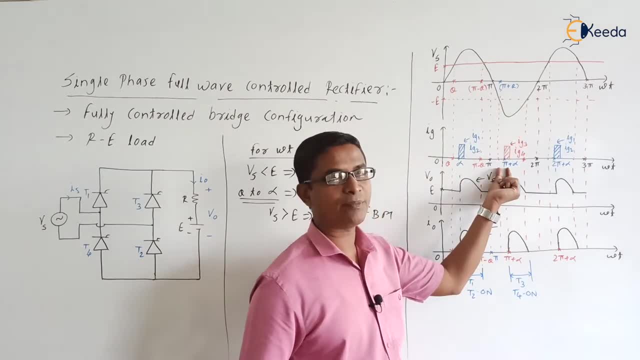 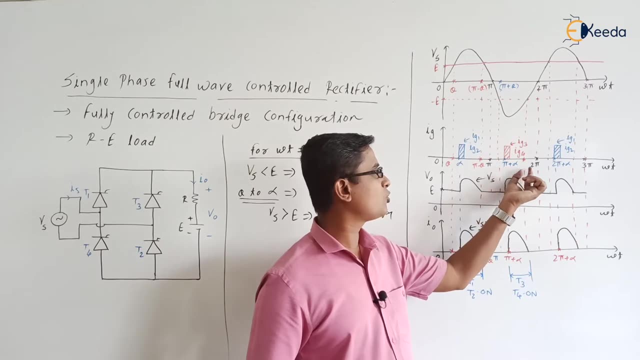 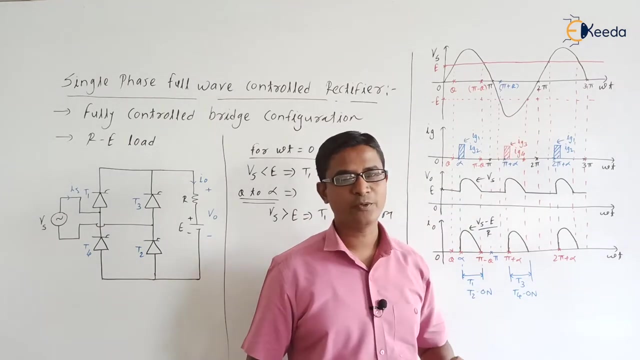 pi. sorry. pi plus theta to pi plus alpha. from pi plus theta to pi plus alpha, thyristor t3- t4 will be in the forward blocking mode: pi plus alpha till 2 pi minus theta. pi plus alpha till 2 pi minus theta. yes, magnitude of vs is greater than magnitude of e. okay, so thyristor t3- t4 will be in the forward. 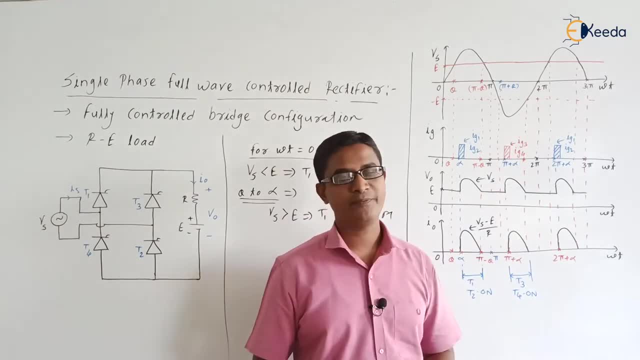 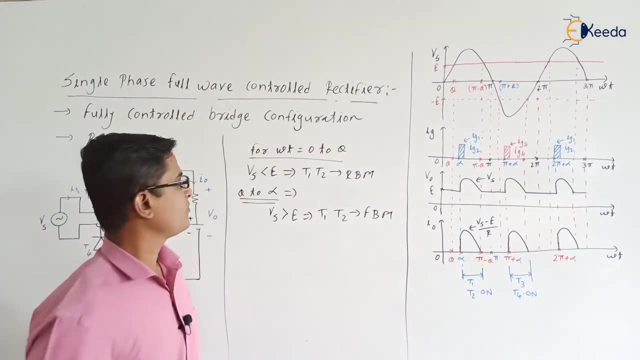 conduction mode. okay, and from 2 pi minus theta to 2 pi t3, t4 will be in the again in the reverse blocking mode. okay, so here we will summarize it. how will be the modes of operations of the thyristors t1, t2, t3, t4? 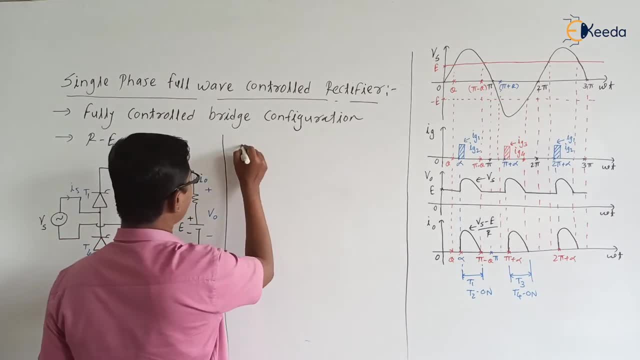 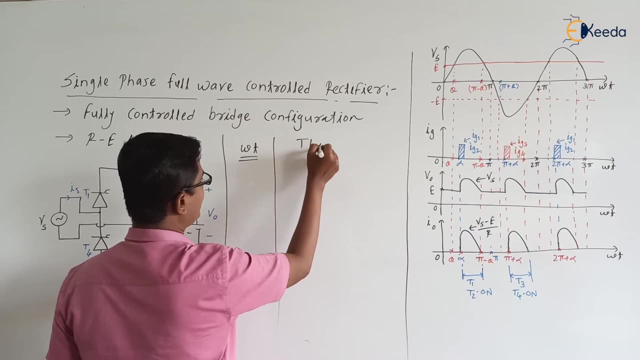 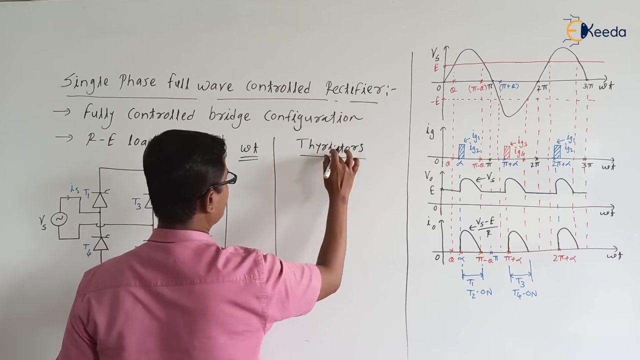 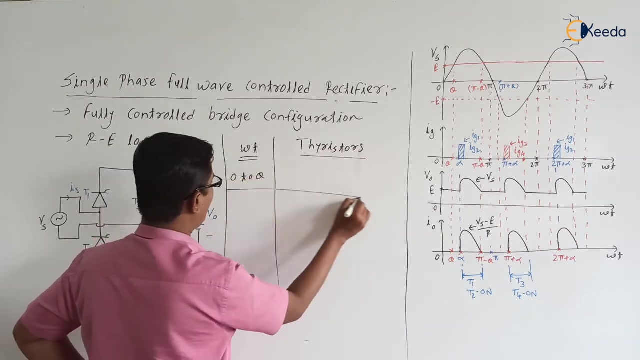 okay. so if you check, i am writing it as a omega t, right next, and thyristors, thyristors, right. so if you check from, omega t is equal to 0 to theta. 0 to theta, okay, for 0 to theta. yes, vs is less than e, okay, so 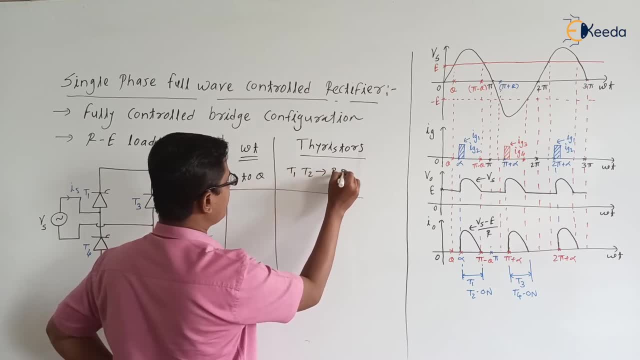 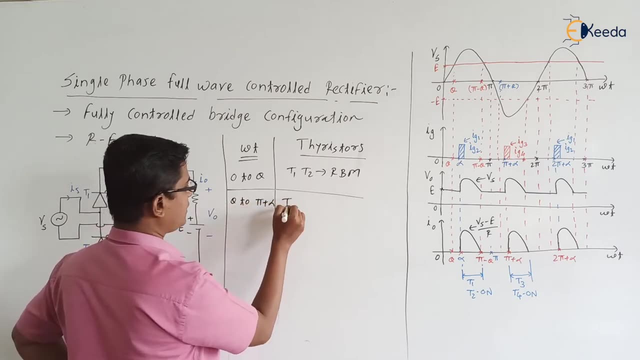 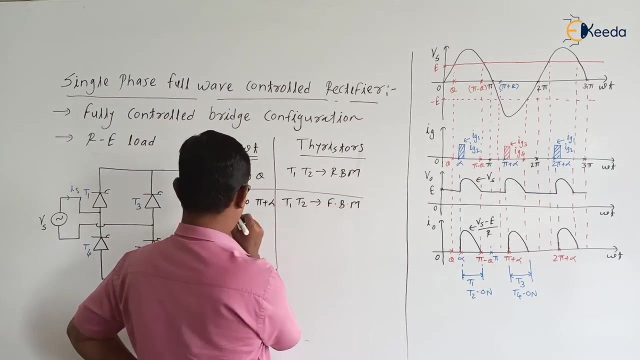 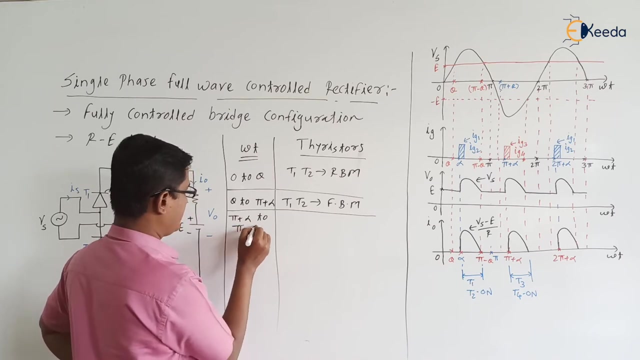 thyristor t1- t2 will be in the reverse blocking mode: right theta to pi plus alpha. theta to pi plus alpha. yes, t1- t2 will be in the yes forward blocking mode from pi plus alpha to pi minus theta. thyristors t1- t2 will be in the forward conduction mode. 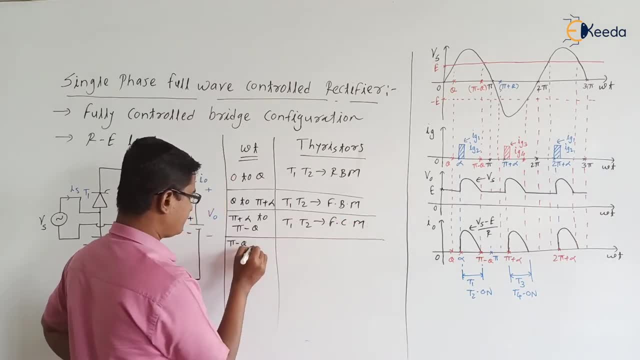 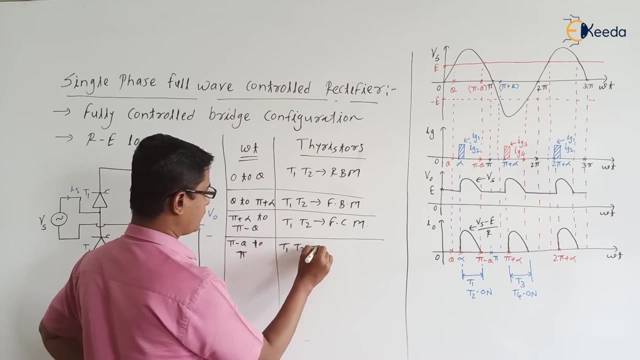 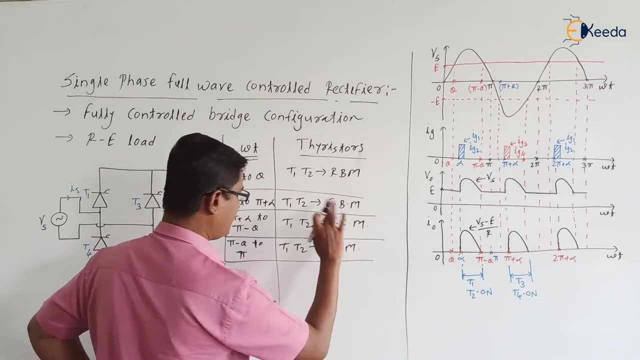 right next: from pi minus theta to pi. pi minus theta to pi- yes. thyristor t2- t2- yes. will be in the again reverse blocking mode because vs is less than e right. similarly, we can write for: thyristor t3- t4- okay. from pi to pi plus theta. thyristor- t3- t4- yes. 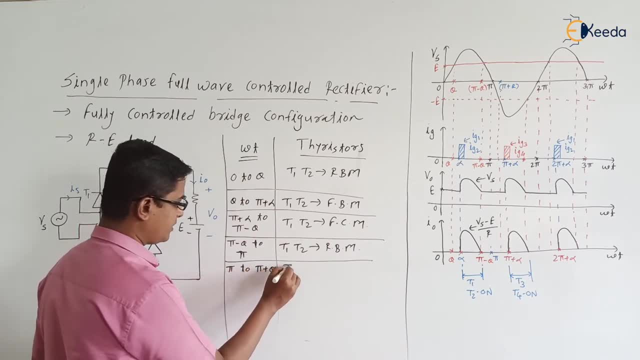 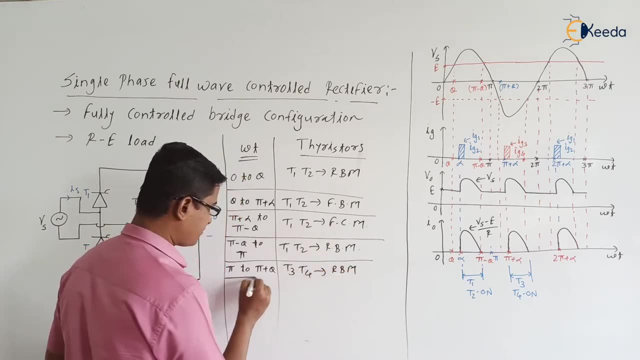 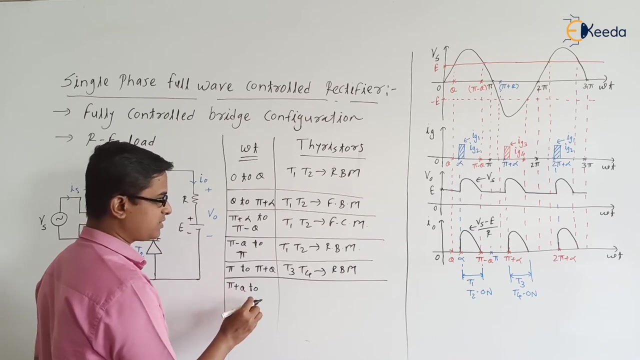 pi to pi plus theta. t3- t4 will be in the reverse blocking mode right next: pi plus theta, pi plus theta to pi plus theta to pi plus alpha, pi plus theta to pi plus alpha. yes, thyristor t3- t4 will be in the 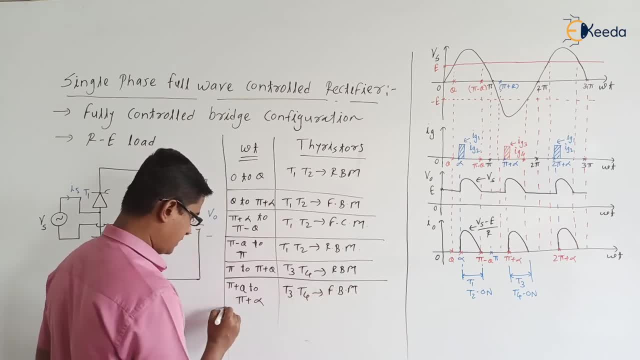 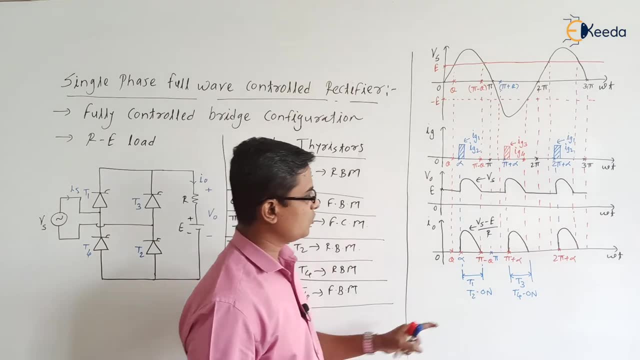 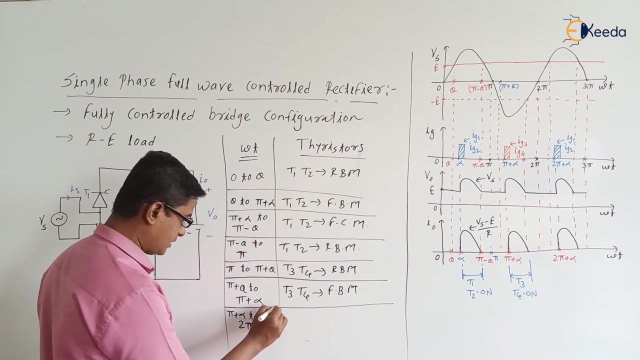 forward blocking mode. okay. next, from pi plus alpha to yes, pi plus alpha to 2 pi minus theta. this instant is 2 pi minus theta, okay, so 2 pi minus theta during this instant. t3, t4 will be in the forward conduction mode. and last, from 2 pi minus theta to 2 pi. 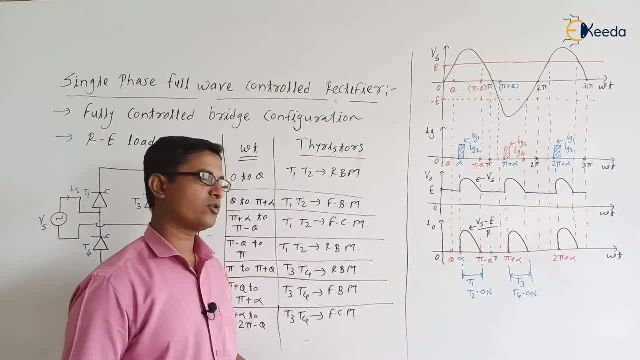 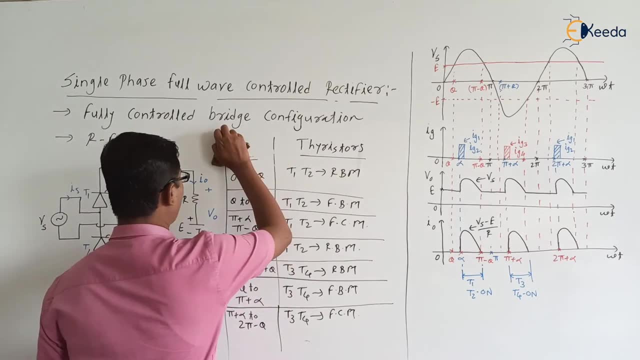 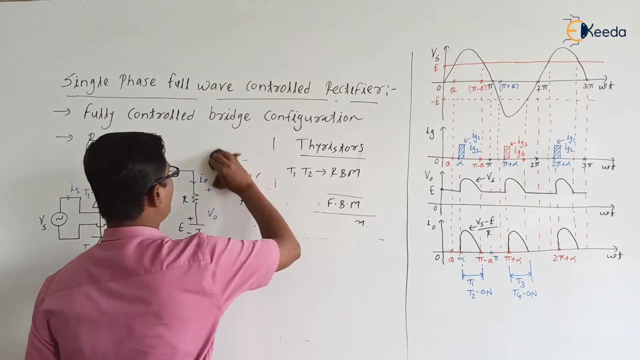 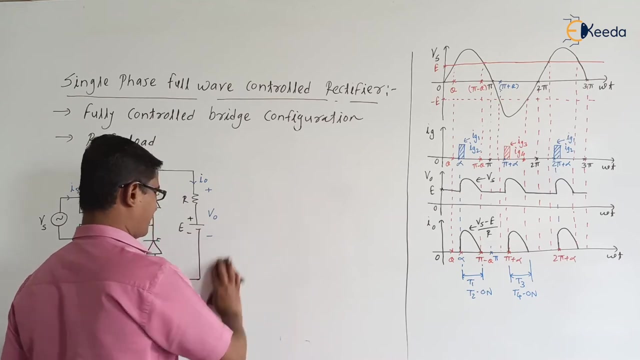 2 pi minus theta to 2 pi s, the t3, t4 will be in the reverse blocking mode. are you getting the point? okay, so from this now we are going to discuss the circuit operation. okay, circuit operation. so from omega t is equal to 0 to alpha. from omega t is equal to 0 to alpha. yes, in the 0 to alpha. 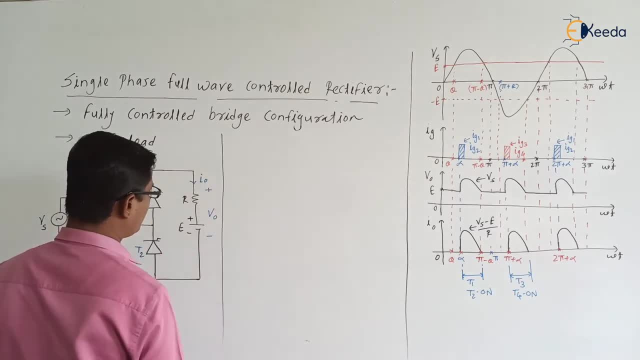 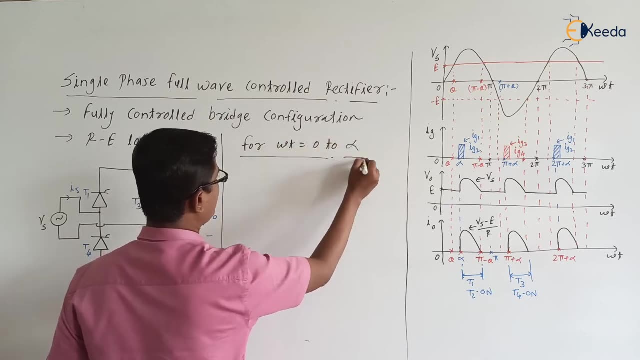 again we are having the two intervals 0 to theta, theta to alpha. okay, so for omega, t is equal to 0 to alpha. yes, 0 to alpha means we have not applied the gate signal to thyristor. okay, so here all the four thyristors will be in the off state. 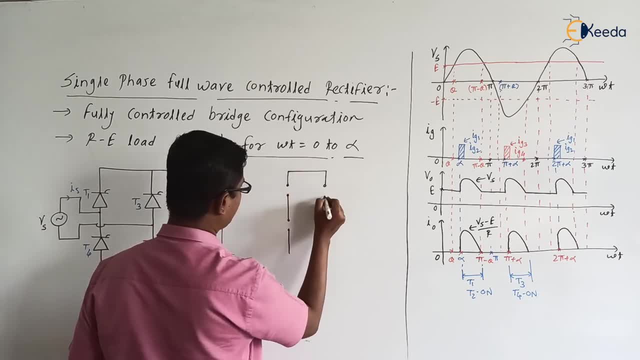 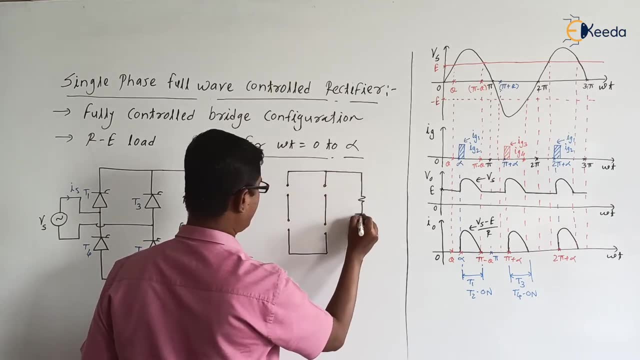 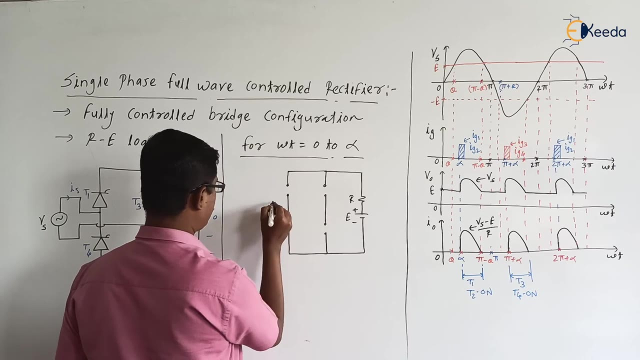 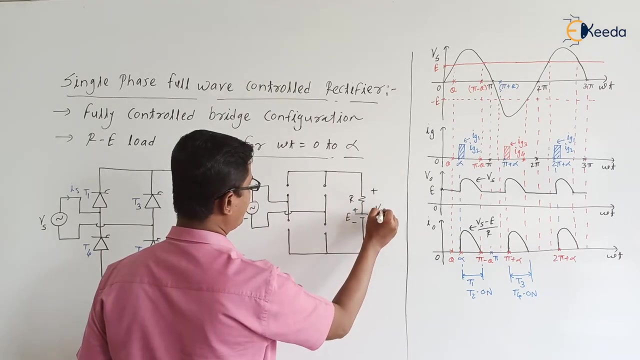 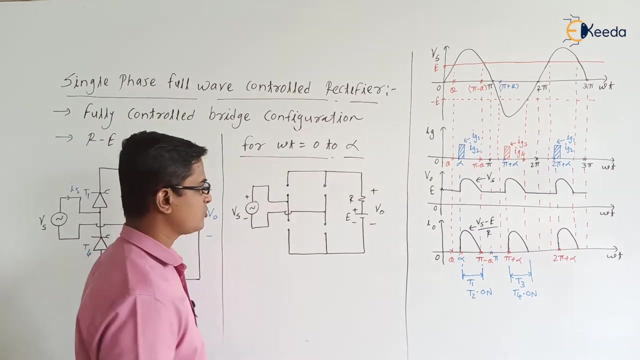 load is re load right. supply here we are having. supply voltage is positive, okay. so what is the v0 now? if all the four thyristors will be in the off state, okay, t1, t2 will be in the reverse blocking mode- okay. so what is the v0 we can? 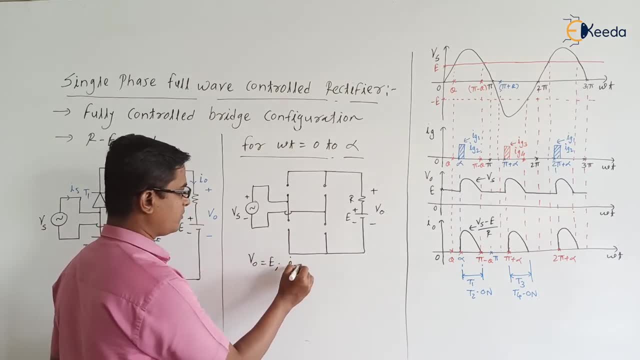 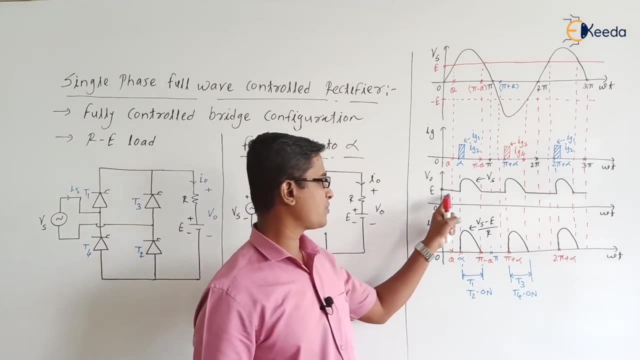 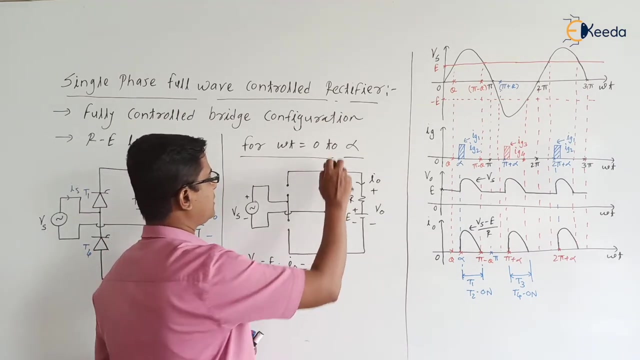 write it as a v0 is equal to e. okay, what is i0? if you check i0, i0 is equal to 0 ampere. okay. so 0 to alpha, v0 is equal to e and i0 is equal to 0, okay, next, from alpha to pi minus theta. for omega, t is equal to alpha to pi minus theta. 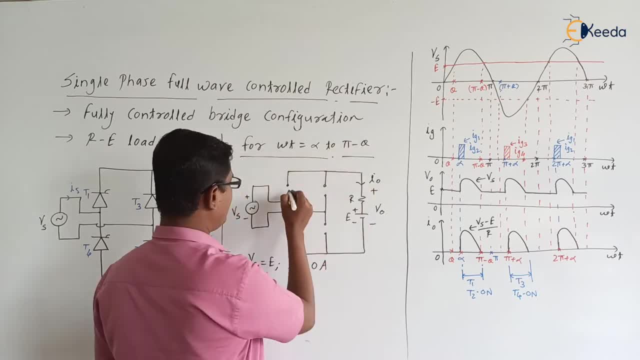 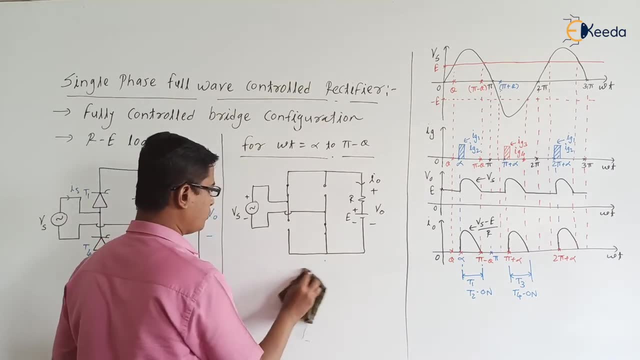 alpha to pi minus theta. yes, what will happen? these two thyristors will be in the on state now. okay, so current will be flowing from v s to i0. okay, so current will be flowing from the on state to e and i will write it as v 0. okay. 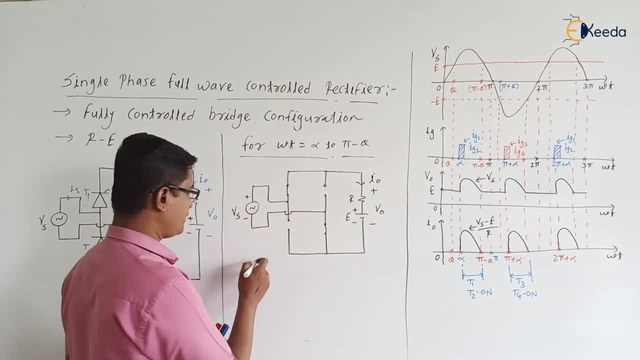 V s T 1, load T 2, and again back to the V s right. V S T 1, load T 2, and again back to the V s. so what is the v0? yes, we 0 will be same a that of the supply voltage, right. and what is the i0? 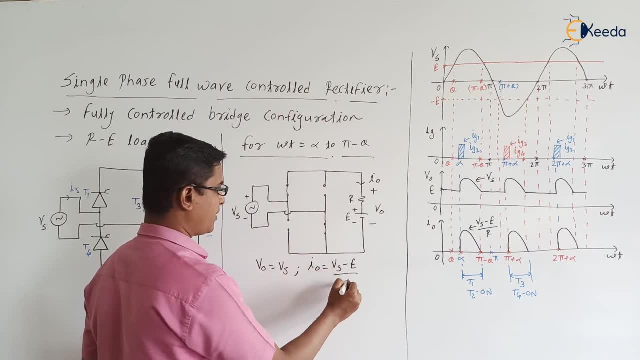 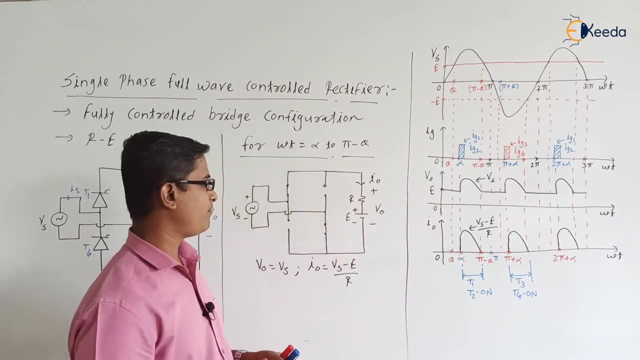 yes, we got that. I 0 is equal to v s minus e by our. okay. i 0 is equal to v s minus e divided by R. okay, so we s minus a by r. pi minus theta. from pi minus theta to pi. what will happen from omega t is equal to pi minus theta to. 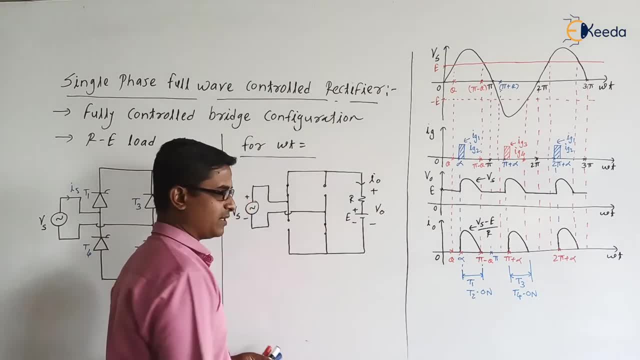 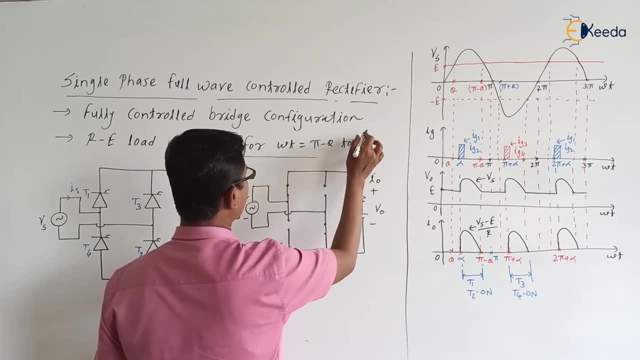 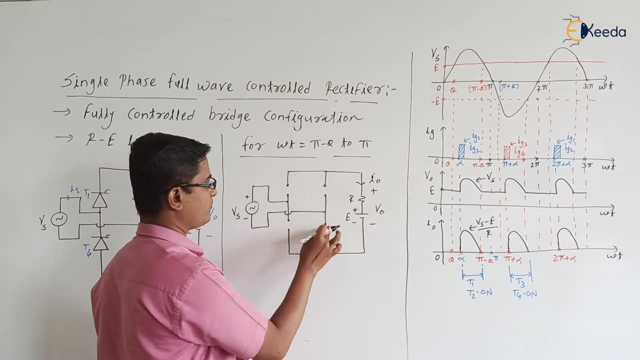 pi, omega t is equal to pi minus theta till pi, pi minus theta to pi. so during this interval, if you check, yes, pi minus theta to pi, e vs is less than e. okay, so again, our thyristors will be in the off state only. okay, so thyristors are in the off state. so what is the v0? v0 is equal to e only, and. 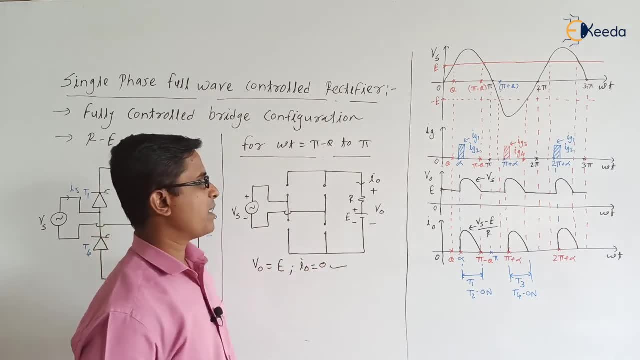 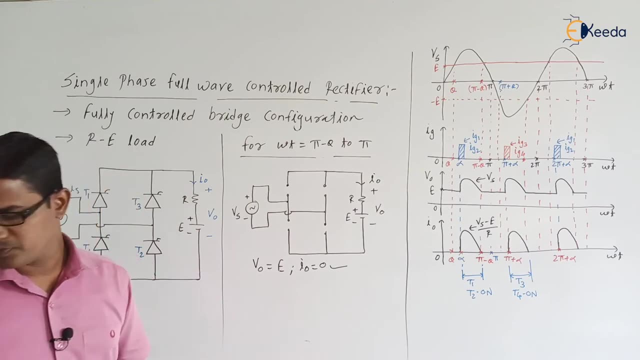 what is i0? i0 is equal to 0. okay, so pi minus theta to pi. if you check, v0 is equal to e, i0 is equal to 0. are you getting the point, okay? next, from pi to pi plus, alpha for omega t is equal to pi to pi plus. 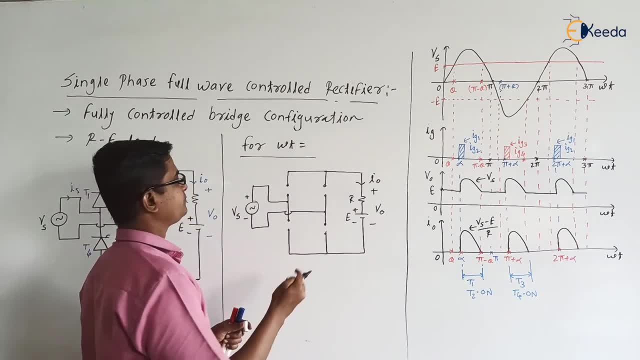 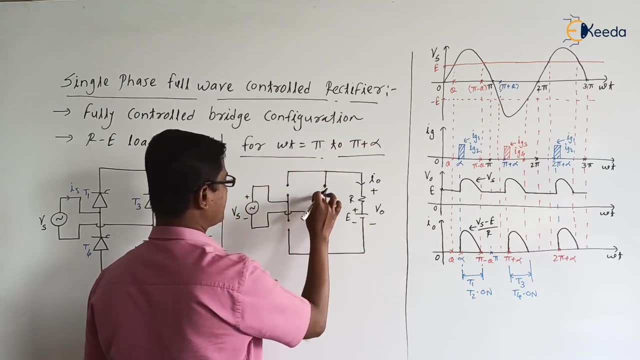 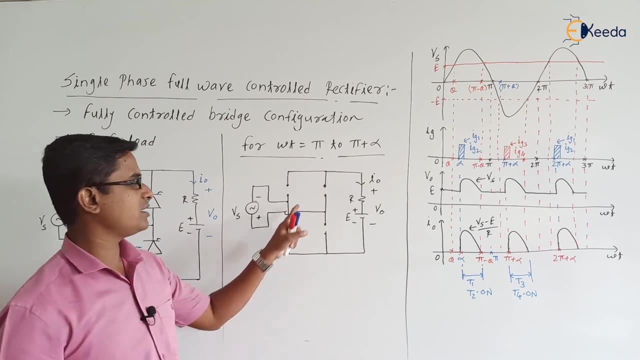 alpha. pi to pi plus alpha. pi to pi plus alpha. yes, yes, during this interval, yes, supply voltage is reversed. okay, so here it is a minus and here it is a plus. okay, during pi to pi plus alpha: yes, we have not applied the gate signal to t3- t4. 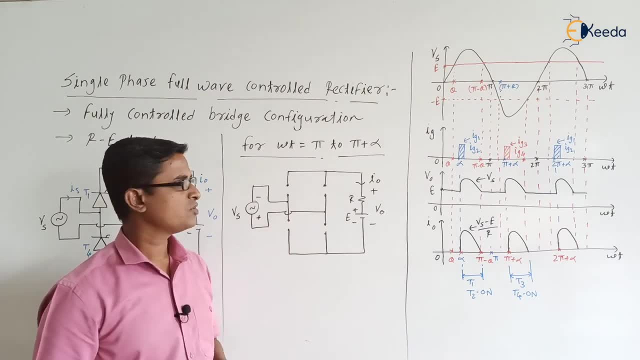 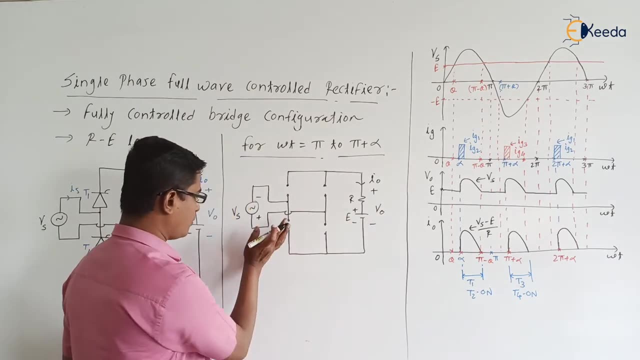 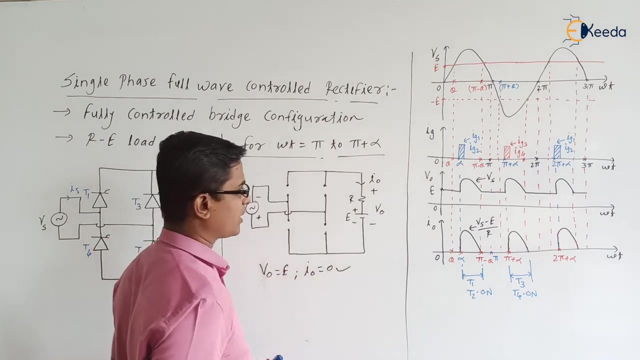 okay. and t1, t2- they are already in the reverse bias mode, okay. so what is the output voltage? yes, if you check, current will not flow from source towards the load. yes, output voltage: v0 is equal to e. only v0 is equal to e. and what is i0? i0 is equal to 0. okay, 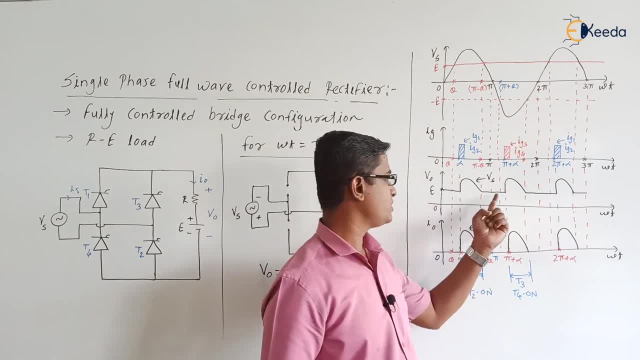 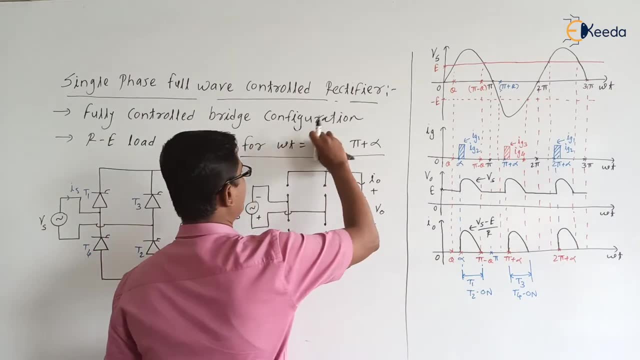 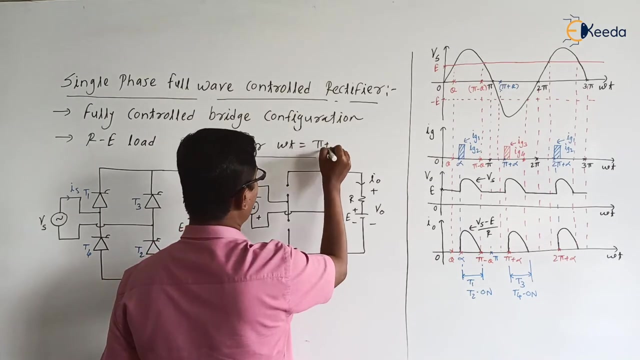 yes, here you are getting the point. okay. so pi to pi plus alpha, v0 is e, i0 is 0. okay, next, from pi plus alpha to 2 pi minus theta, from pi plus alpha to 2 pi minus theta, from pi omega t is equal пока. 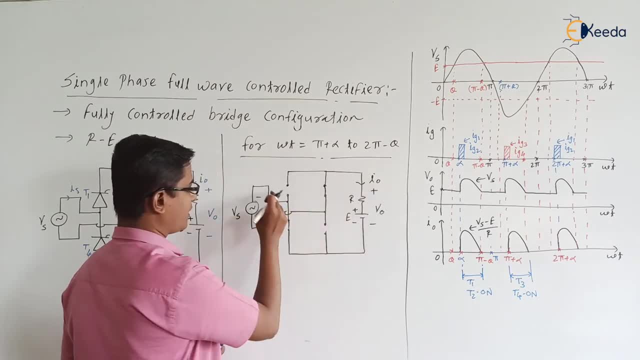 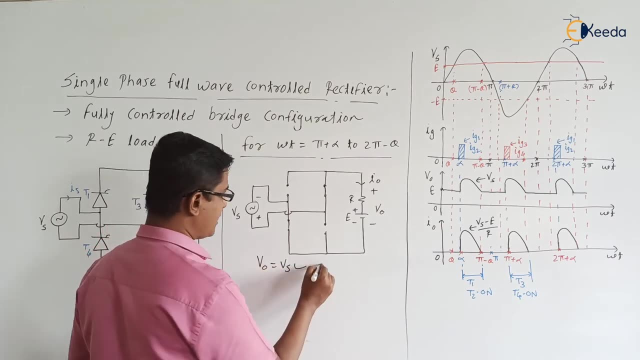 so if you are in the on state, current will be flowing from vs t3, load t4 and again 5 plus alpha, 2 pi minus theta. so if you are in the on state, current will be flowing from vs t3, t4elia back to the vs. okay, what is the v0? v0 will be supply voltage right. it is a positive right. i0. 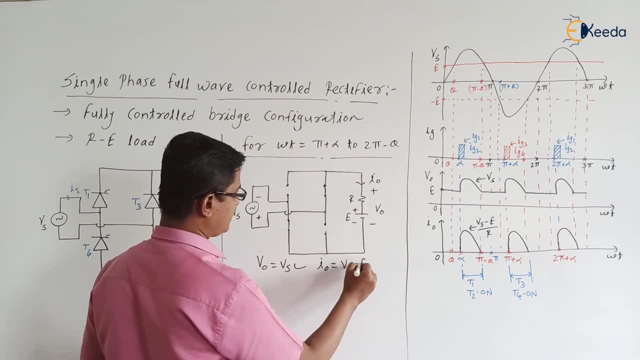 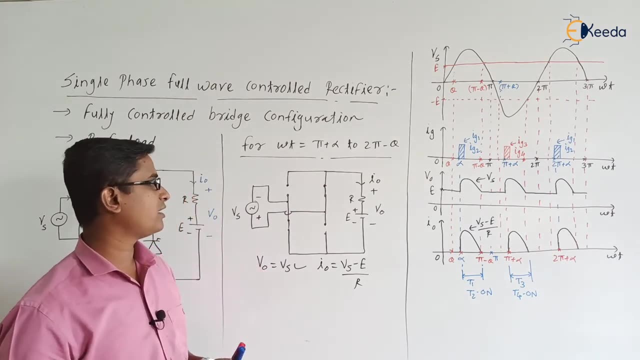 i0 is equal to yes vs minus e divided by r. you can apply kvl. you will be getting this expression. i0, okay, is equal to vs minus e by r. so, from pi plus alpha to 2 pi minus theta- yes, we are having this expression, okay. next, from 2 pi minus theta to 2 pi. what will happen from 2 pi minus theta?